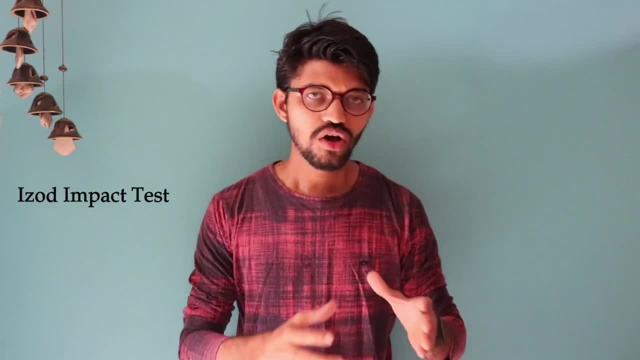 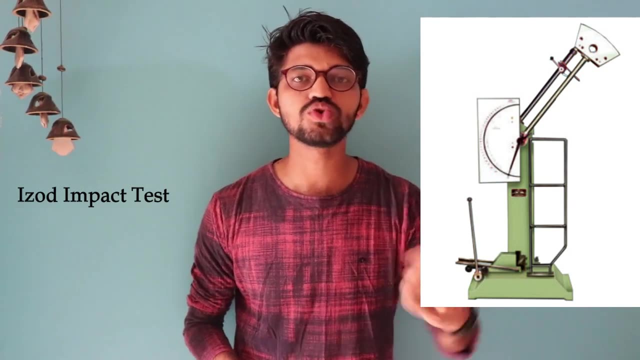 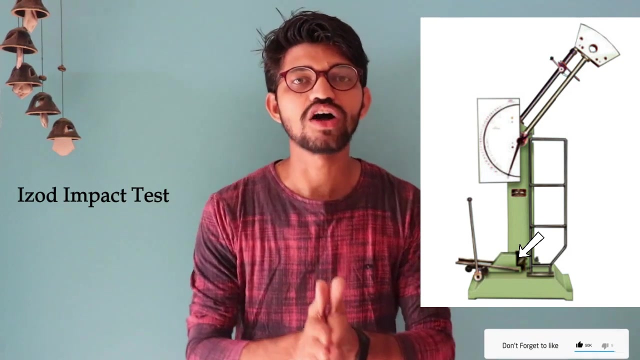 let's take first of all the Izod impact test. so over here you can see, this is the impact testing machine, which is having a pendulum type hammer connected to a scale, and on the tower, on the just below that the hammer, there is like a anvil, and upon that anvil or specimen will be kept. so in the case of Izod, 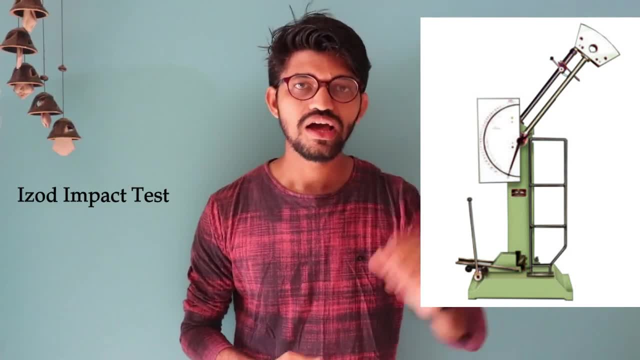 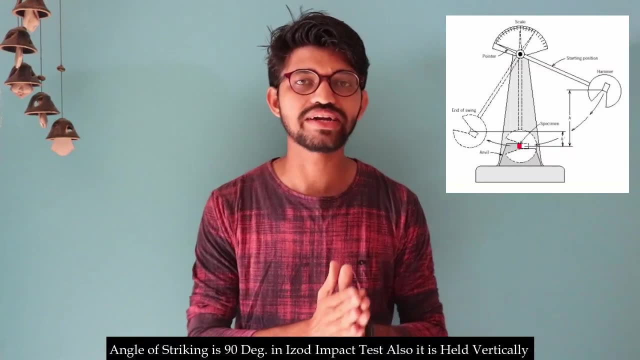 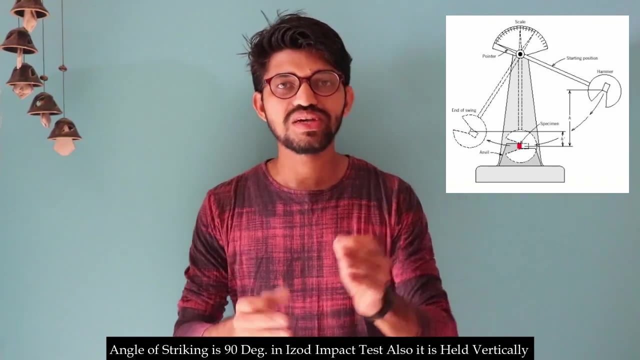 impact test, this particular pendulum hammer is having a scale and it is set to a portion of a 90 degrees in case of the Izod impact test. so the you know, the hammer is set at the scale of the 90 degrees, which is totally perpendicular to the specimen, the specimen held vertically. so the 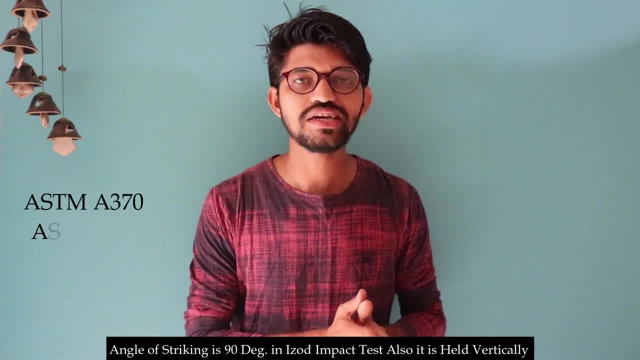 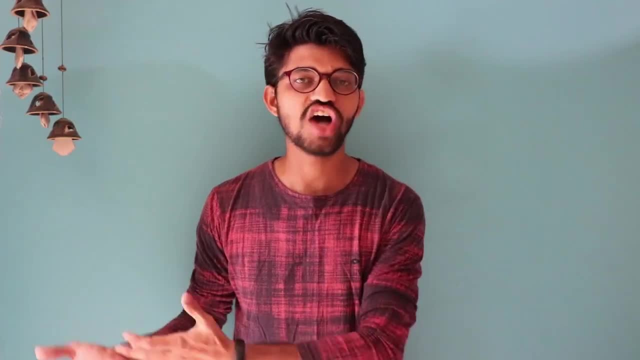 specimen belongs to the specifications of the ASTM A370 or else ASTM E23. so that particular standard is for the both of the test, that is, for the Izod, as well as the for the sharp impact testing. so over here in case of the Izod impact, 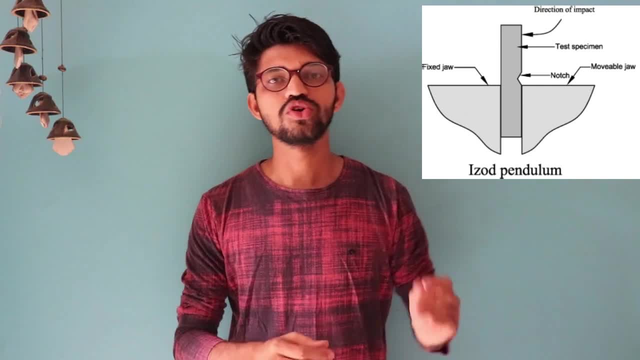 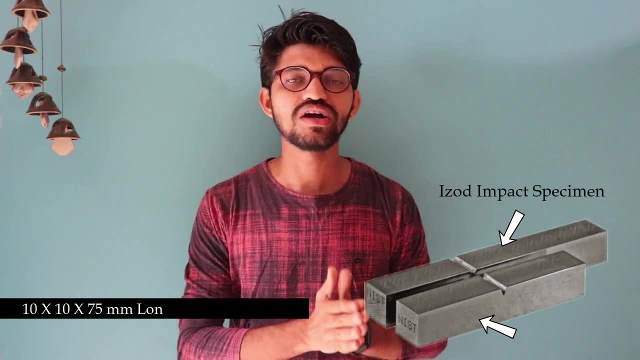 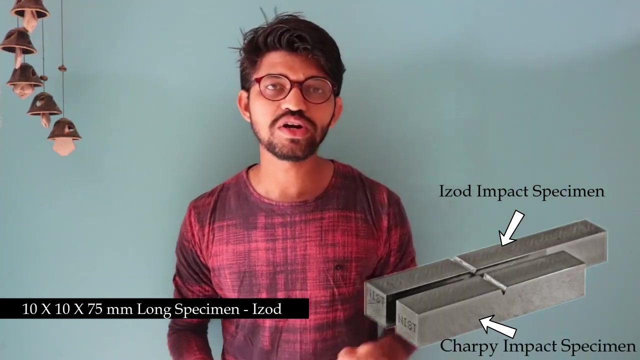 test the specimen held vertically, such that you know the specimen will be having the specification of the, which is having a 10 mm square and will be having a 75 mm long in case of the Izod impact test. so these are the standard specification of the specimen also this: 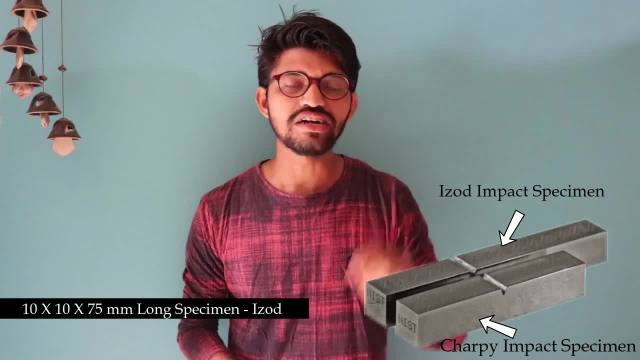 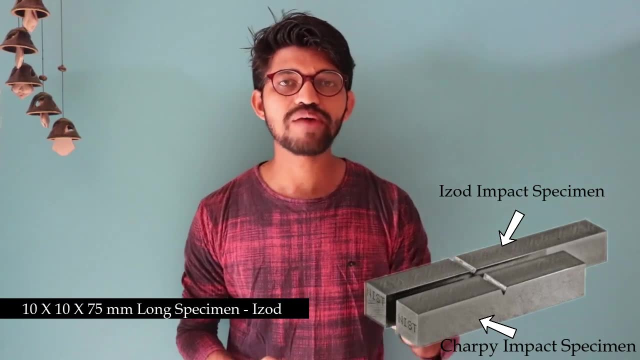 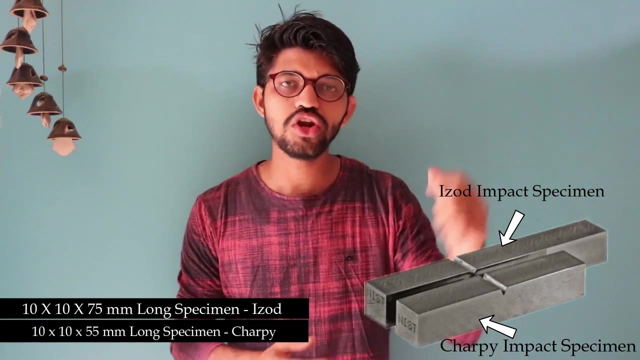 particular specimen is having a V notch over there in the center which is 2 mm deep and having a 45 degree of angle. so that is the, you know, that is the required parameters over here in Izod impact test. in the sharp impact test the specimen will be at the same, having the V notch and a 2 mm deep thickness. but 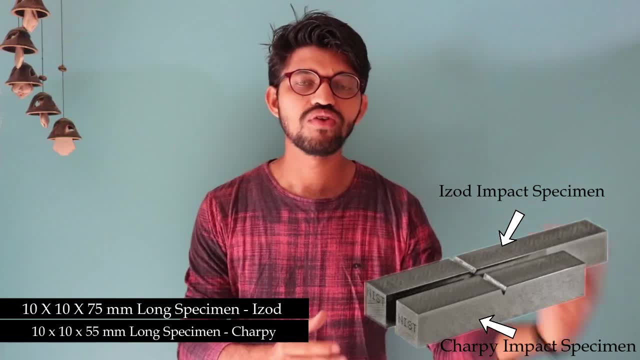 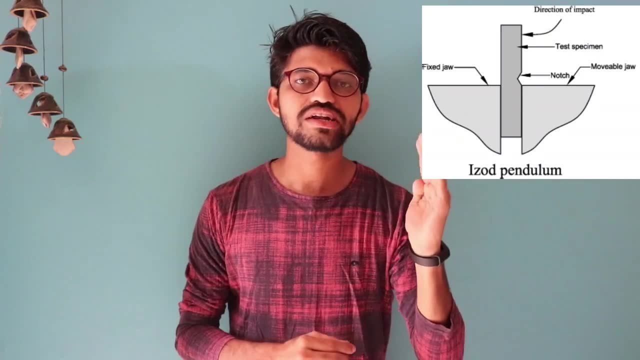 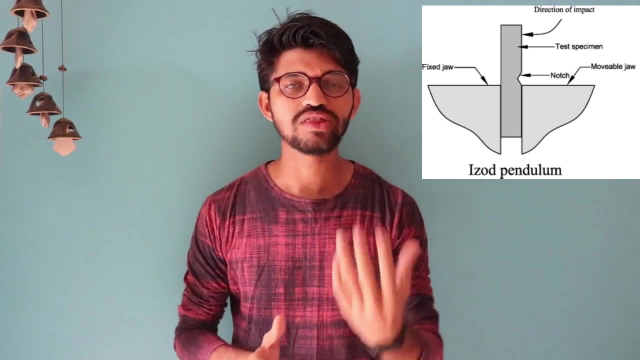 the length of the specimen will be of 55 mm instead of 75 mm. so, moving ahead next, this specimen is held at vertically, such that, you know, such that that particular, like the V notch, is facing towards the hammer. so it is held on the anvil, the 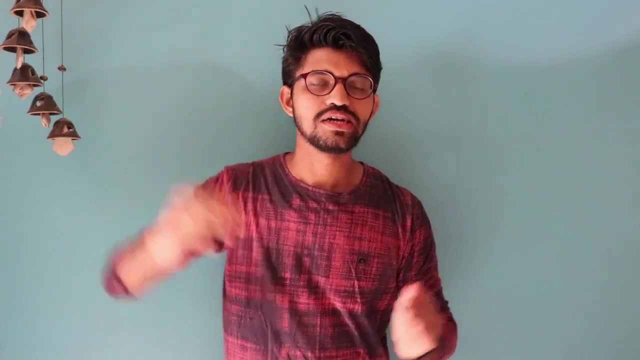 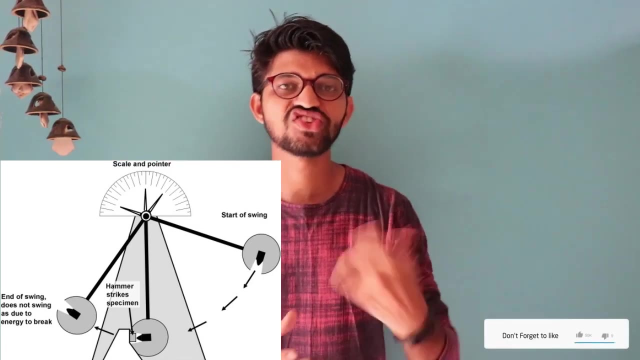 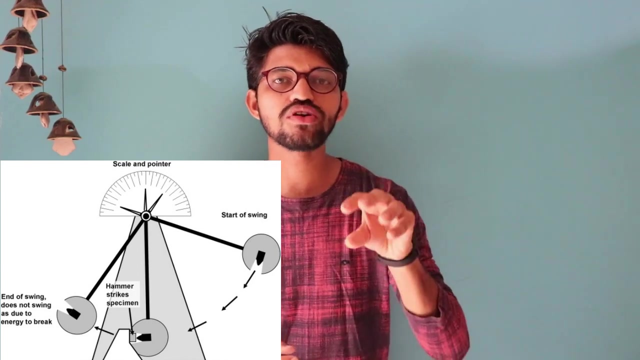 specimen is held on the anvil and then the hammer is released, so that the hammer will get strike on the specimen at the angle of 90 degree. so before that striking, you know the initial amount of the. that is the potential difference in the hammer. that is nothing but the amount of the energy which is there. 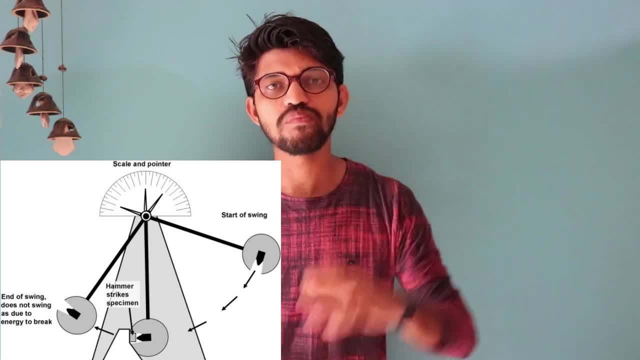 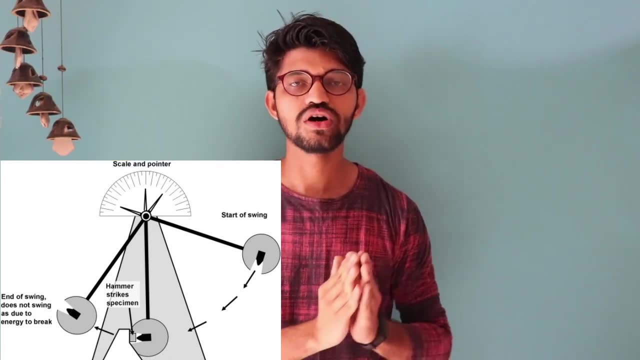 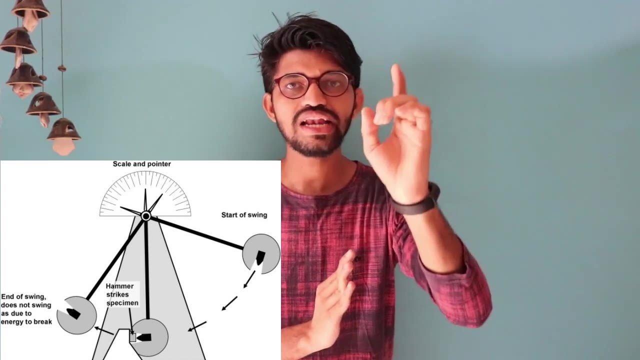 inside the hammer that is noted down from the scale which is connected to the your hammer. and then hammer is released and it gets strike on your work piece, your specimen, so that the- you know the specimen will get deformed actually, and on the after the striking, the scale gives the another mean. so you have to. 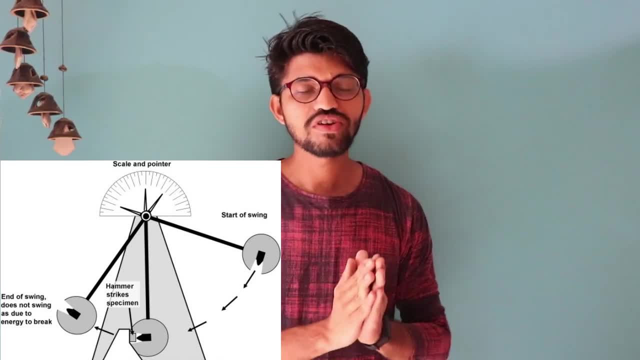 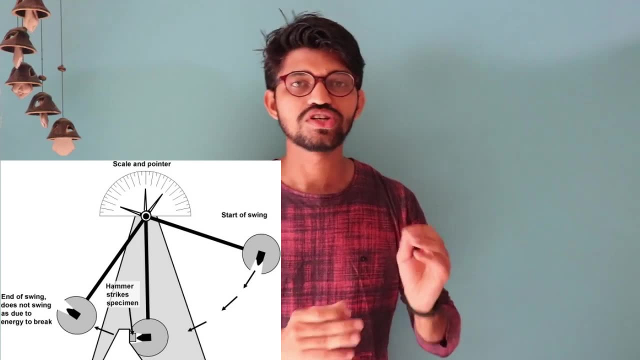 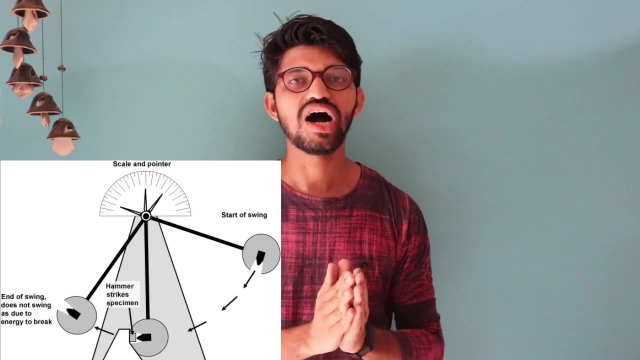 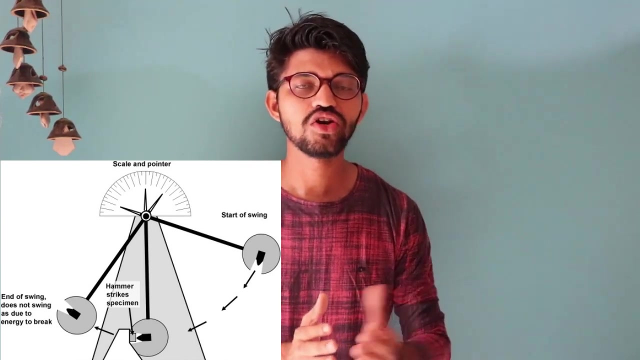 note down that another reading also. so, after striking, the total amount of the energy which is absorbed by the specimen, which is expressed in joules, that is nothing but the initial potential energy in the hammer minus the amount of the energy after striking. so basically we get a value which is nothing. 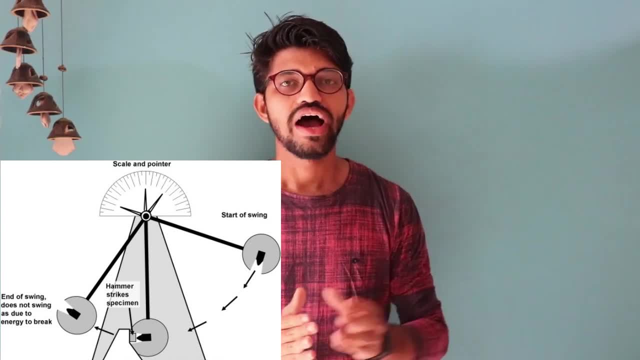 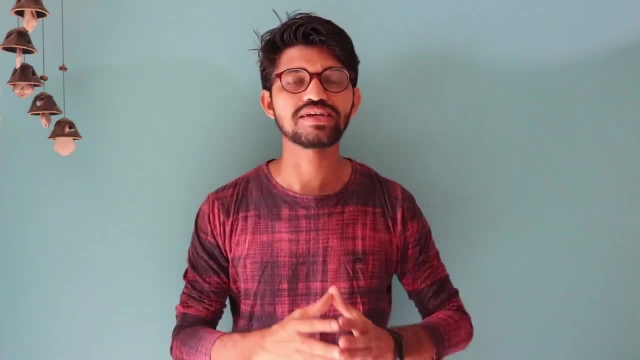 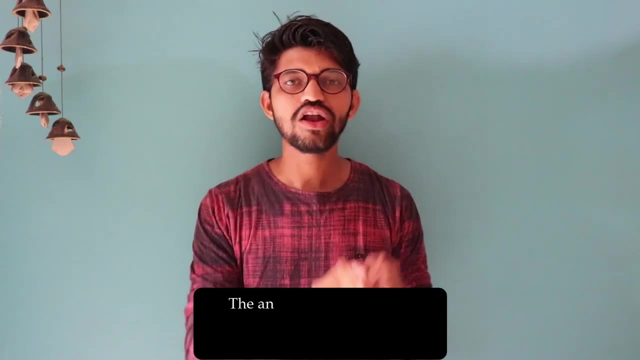 the amount of the energy, which is actually amount of the energy absorbed by your specimen. so that was the whole of the procedure in izod impact test. now let's talk about the sharp impact test. the test is very much similar, except the angle of striking. the angle of striking in izod impact test. 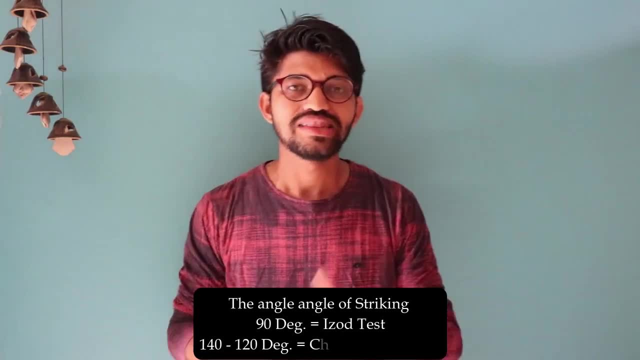 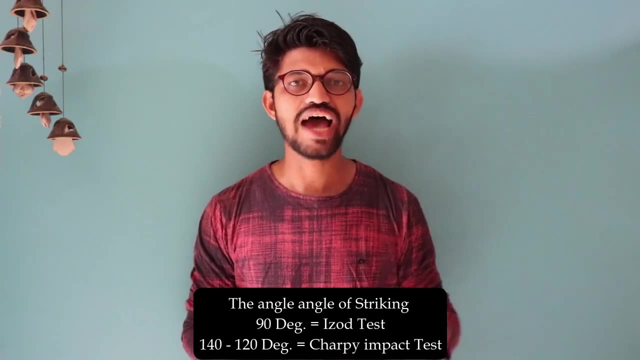 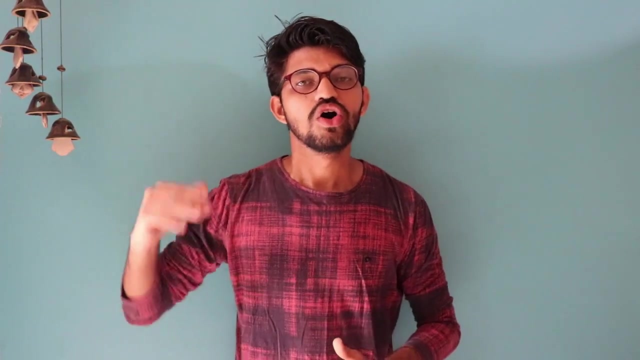 was of 90 degrees, but over here in the sharp impact test, the angle of striking will be of 140 to 120. so moving ahead. next is the- you know, the specimen. the specimen is having a 10 mm square, or else 55 mm long, which is used in izod, and in the chart impact test it will be of the 75 mm long. 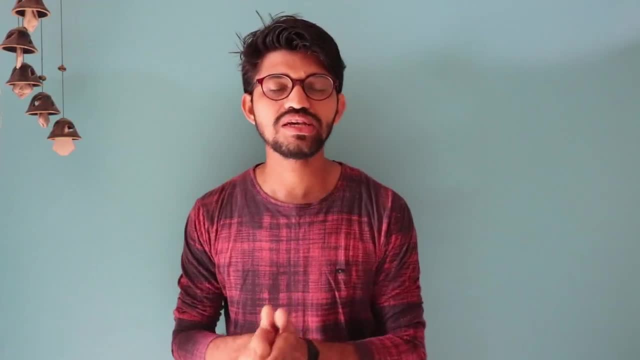 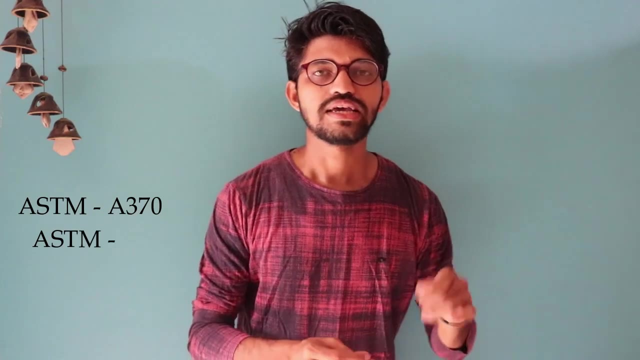 so that is the difference. in the specimen, the standard will be same as that of the izod and the charby, which is nothing but the a370 or else, or else e23, that is astm, american society of testing materials, that is east 23.. also in case of the standard, the standard will be same as that of the 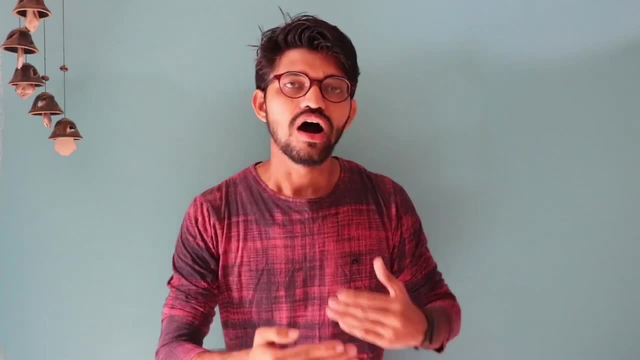 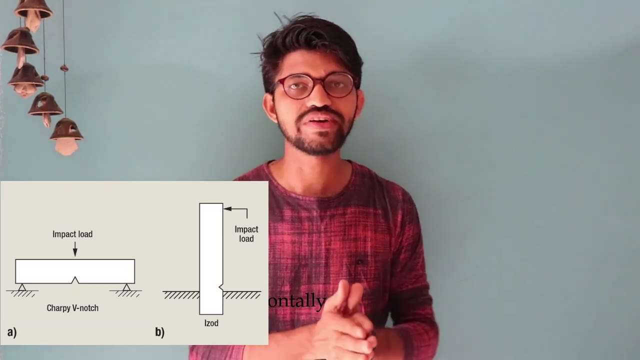 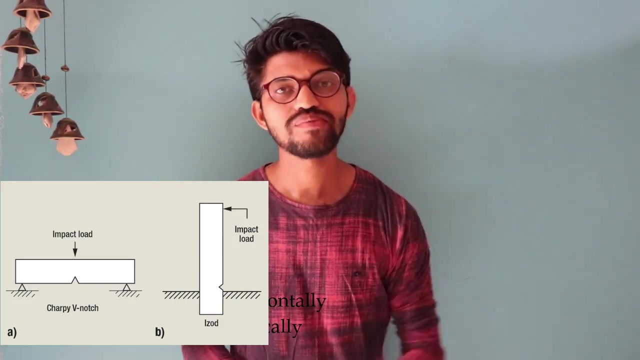 chart impact test. the specimen is held uh, horizontally- horizontally such that you know this particular notch is facing on the opposite side of the uh, your half striking hammer, as that of. in case of the izod impact, the specimen held vertically but over here. in case of the 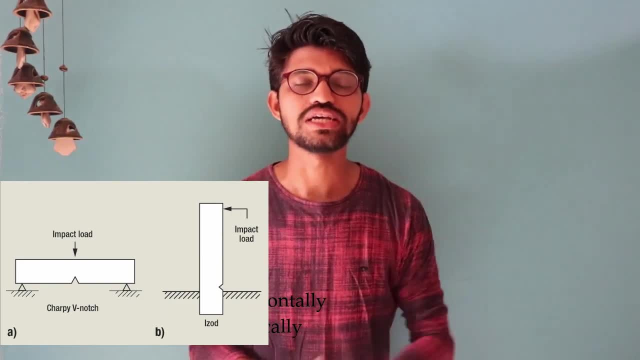 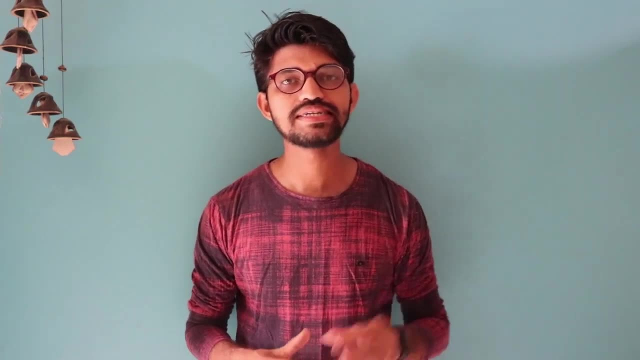 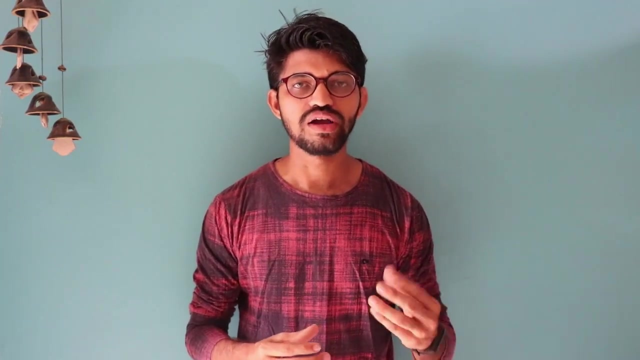 chart impact test, the specimen is held, uh, horizontally. so that is the basic difference between the izod and the chart impact. so now let's understand why these two tests are needed over here. in case of the impact testing condition, so in some of the industries such as the automobile industry,